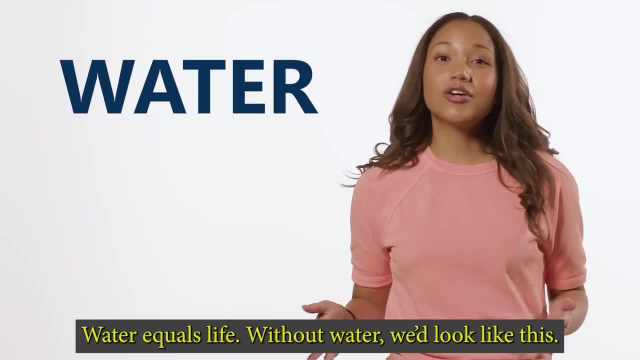 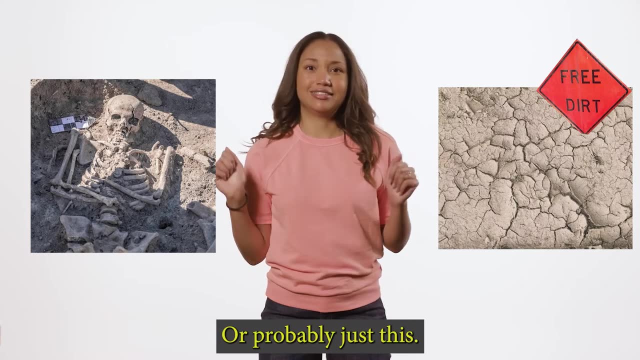 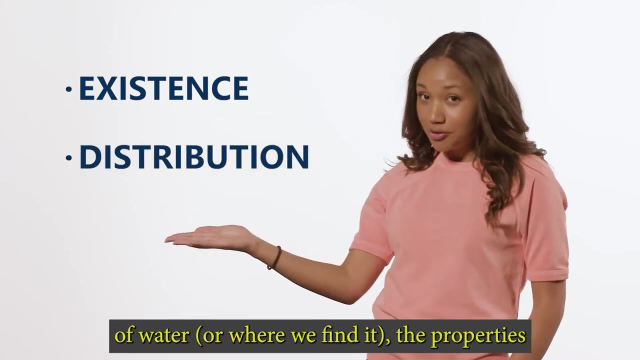 essential natural resources we have on earth. Water equals life. Without water, we'd look like, or probably just like this: When studying hydrology, we look at the existence of water or where it came from, the distribution of water or where we find it and the properties of water. 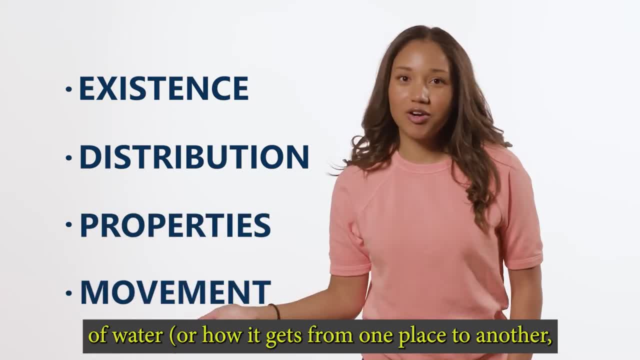 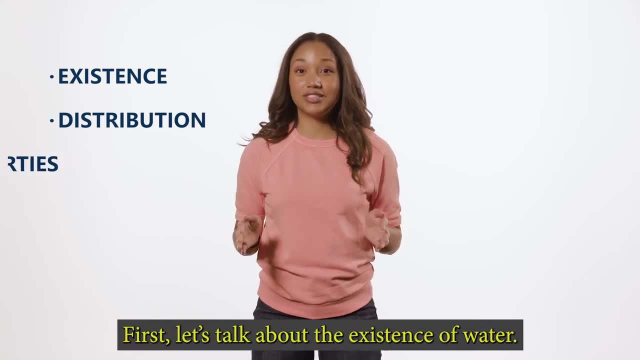 what it's made of Last, the movement of water, or how it gets from one place to another through something called the water cycle. First, let's talk about the existence of water. There are different scientific explanations that tell us where water likely came from. 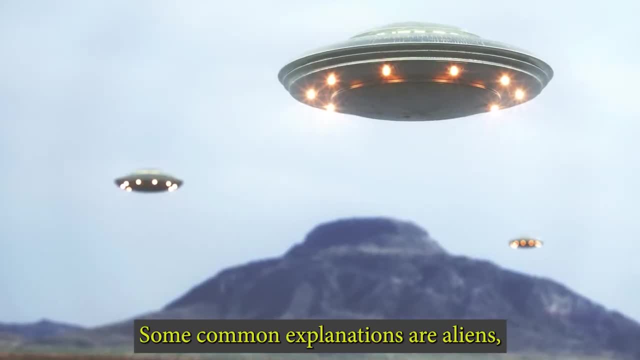 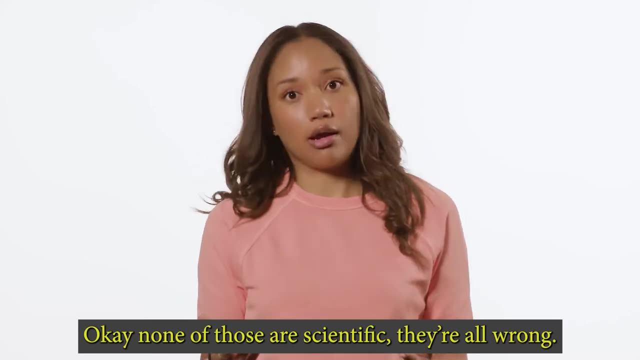 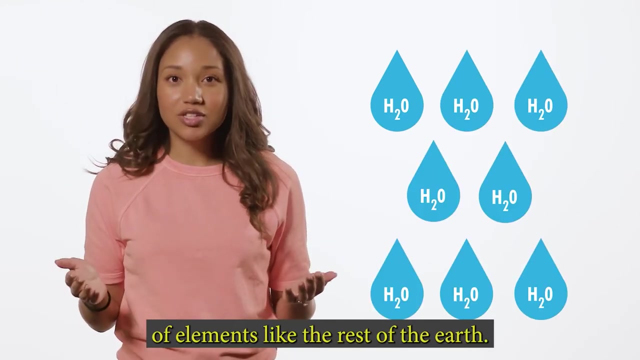 Some common explanations are: aliens, the kitchen sink, smart water bottles. Okay, none of those are scientific. They're actually all wrong. Some of it probably came when the crest of the earth was formed. Water is a chemical made of elements like the rest of the earth As 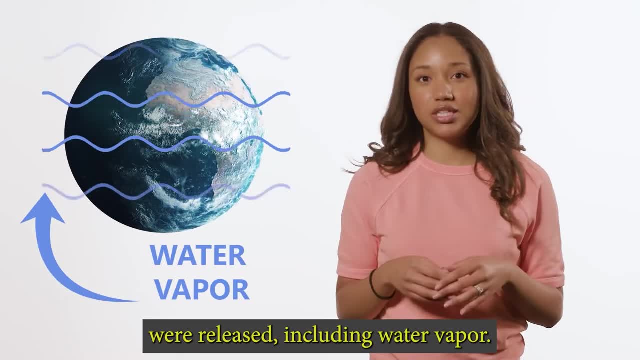 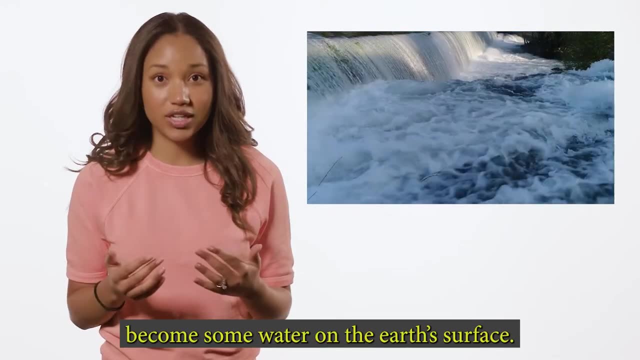 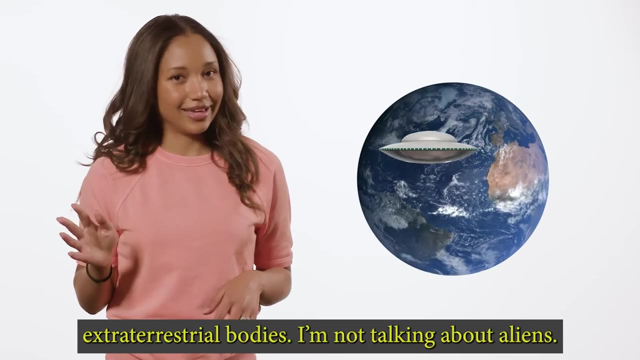 the surface of the earth cooled, some gases were released, including water vapor. This water vapor may have collected together and become some water on the earth's surface. Another source probably came from extraterrestrial bodies. I'm not talking about aliens, That. 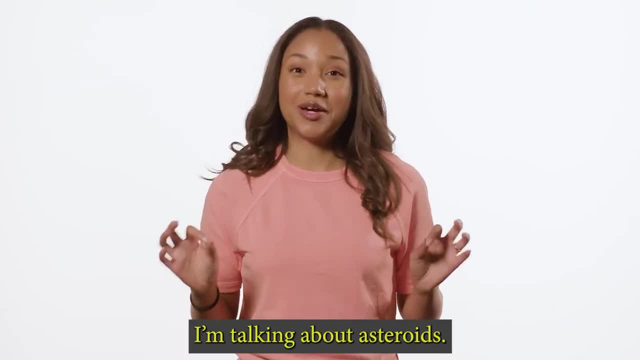 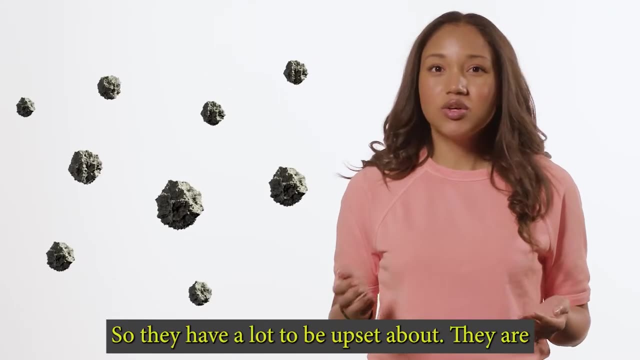 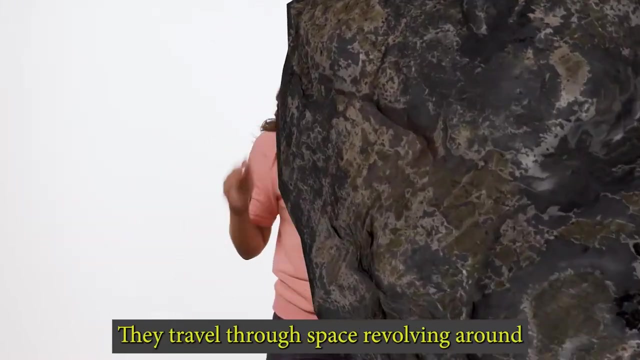 was my first theory, but the scientists said no, I'm talking about asteroids. Asteroids are basically tiny planets that never grew into big planets, So they have a lot of upset about it. but whatever They are- chunks of rocks, minerals and often ice- They travel through space. 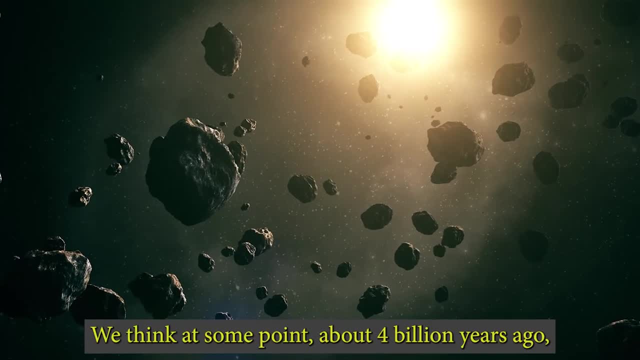 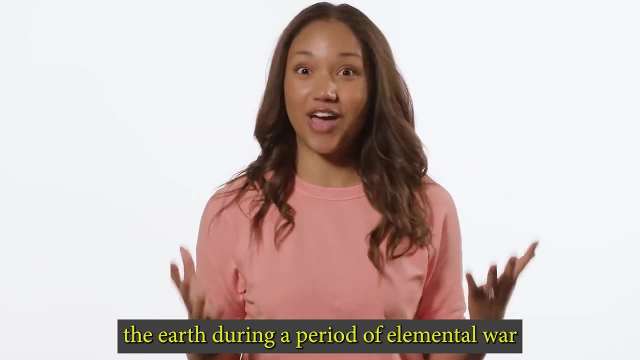 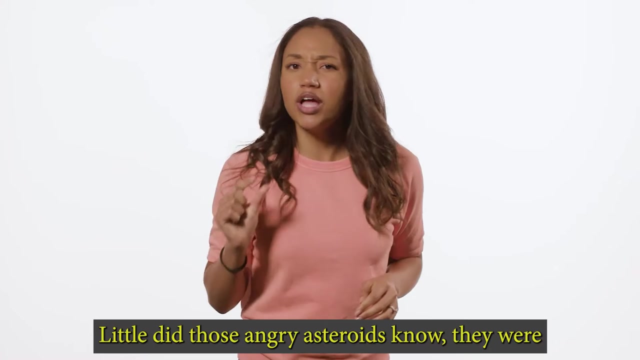 revolving around the sun, like the earth does, We think. at some point about 4 billion years ago, the asteroids formed an alliance and crashed into the earth during a period of elemental war known as the bombardment. Little did those little angry asteroids know they were attacking a hunk of rock that wasn't. 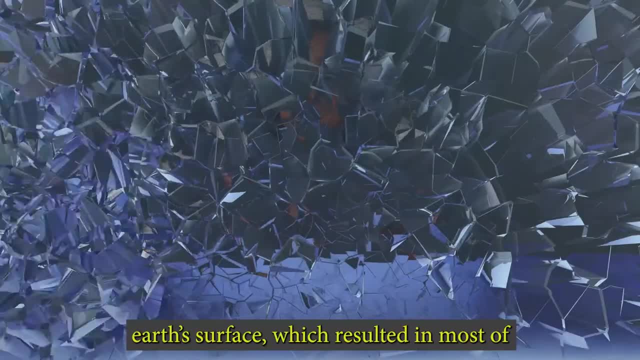 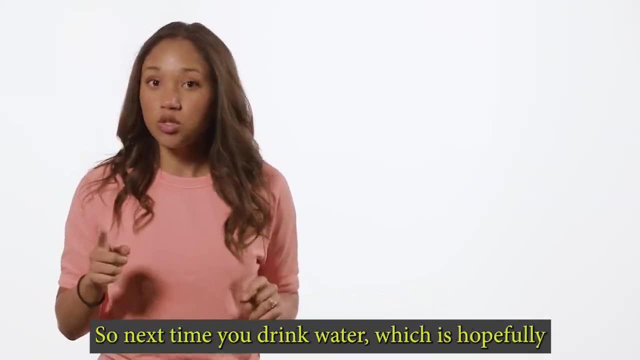 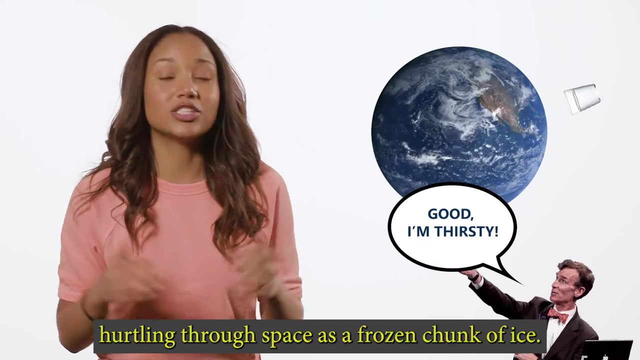 even alive. They likely brought a lot of ice to the earth's surface, which resulted in most of the water here today and therefore life. So next time you drink water- which is hopefully today- you can imagine that little glass of water hurtling through space as a frozen chunk of ice. 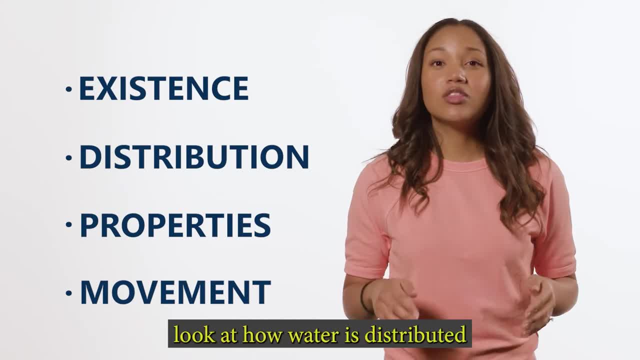 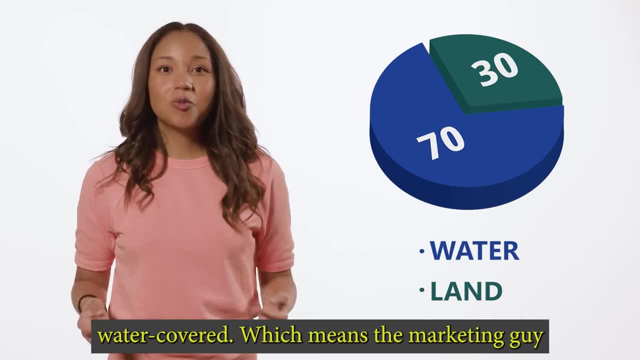 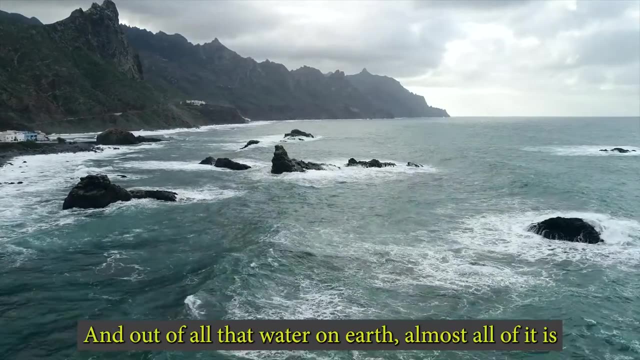 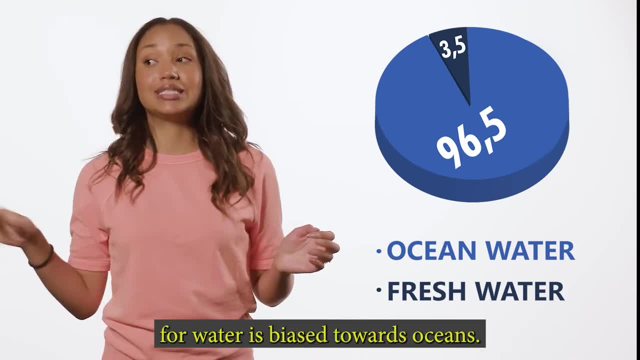 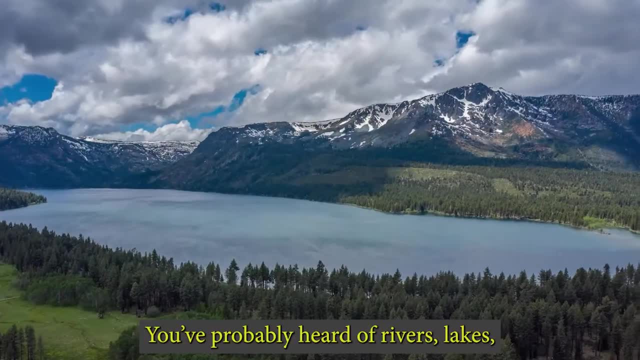 And that's a lot of water, And that's a lot of water And that's a lot of water, Which also means the marketing guy for water is a bias towards oceans. The rest of earth's water is found in various places. You've probably heard of rivers, lakes or smart water. We also have ice caps. 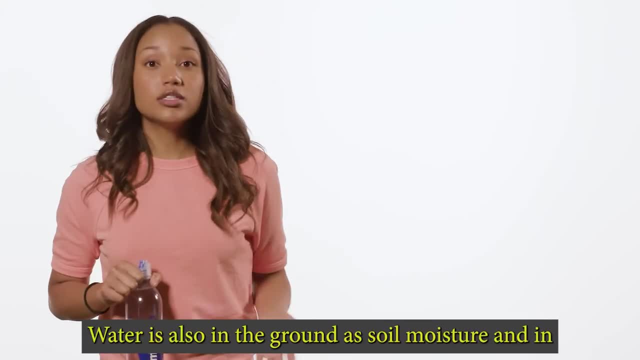 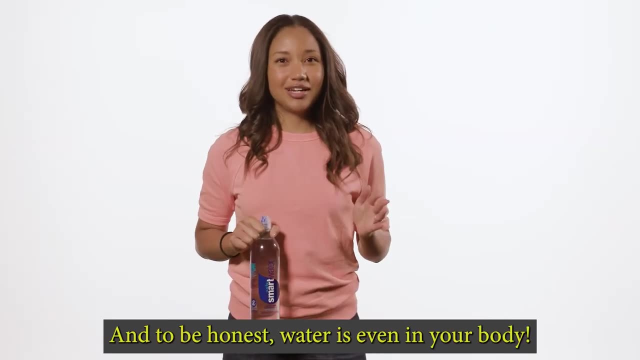 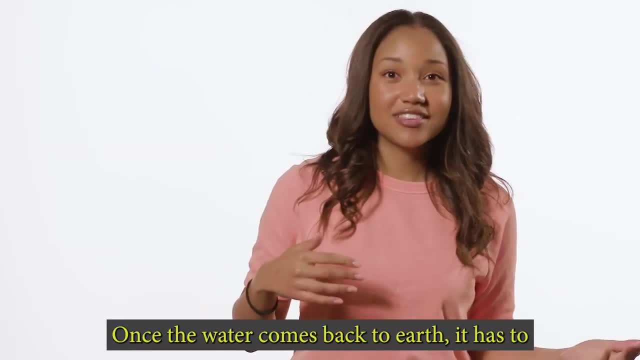 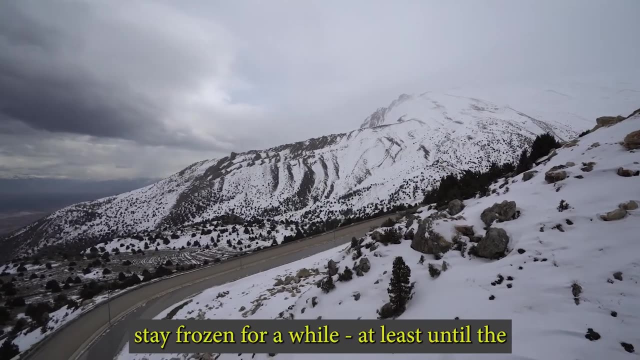 called aquifers, And that's also because of all the smart water. Water is also in the ground as soil, moisture and in underground layers of rocks. Once the water comes back to the earth, it has to go somewhere. If it snowed on a mountain, it might stay frozen for a while, Or until, at least until the temperature rises too long. 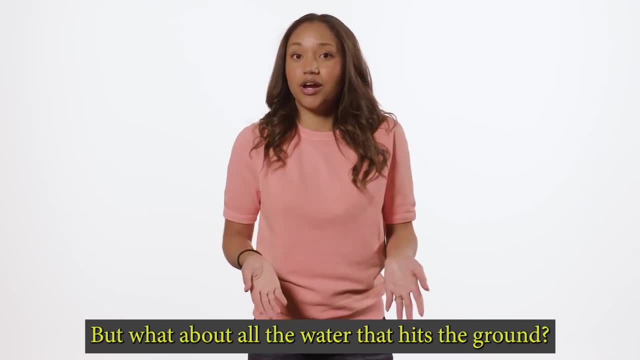 Some precipitation falls back into oceans or lakes. Water cycle shortcut. What about all the water that hits the ground? A lot of this soaks into the soil. In the soil, plant roots absorb the water. A lot of this soaks into the soil. In the soil, plant roots absorb the water. 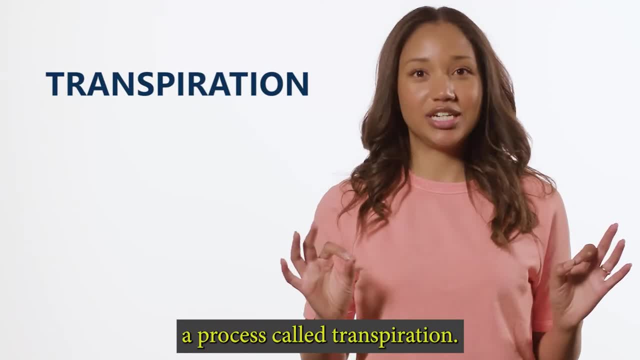 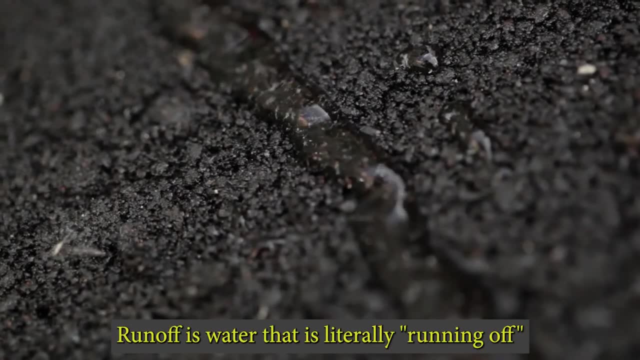 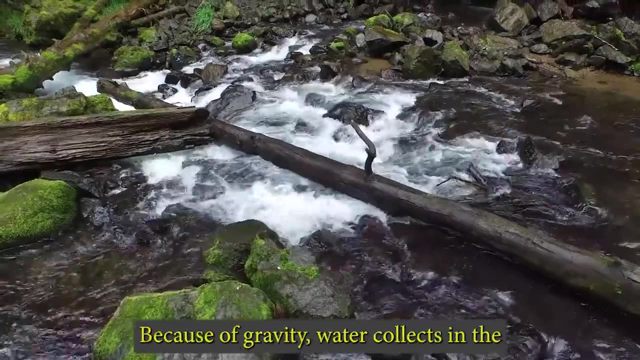 and the plant grows. This is called transpiration. If enough water falls in one place, you have another process called runoff. Runoff is water literally running off from one place of the earth to another. Because of gravity, water collects in the lowest areas Small trickles.